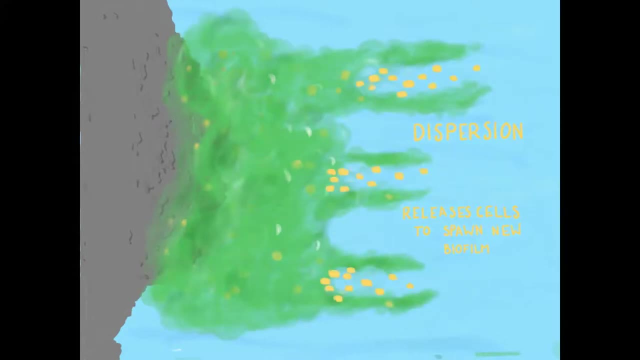 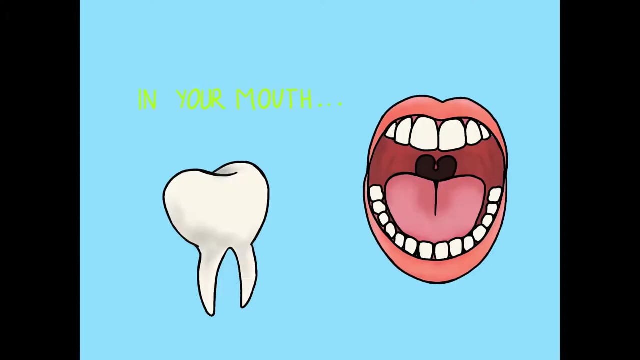 As the biofilm matures, it opens up to disperse cells that can swim to new surfaces and form more biofilms. Then the whole process repeats itself again. Because of their durability, biofilms can form just about anywhere. They can form in your mouth as plaque. 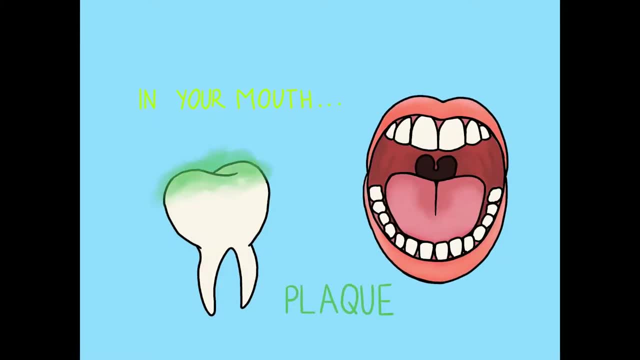 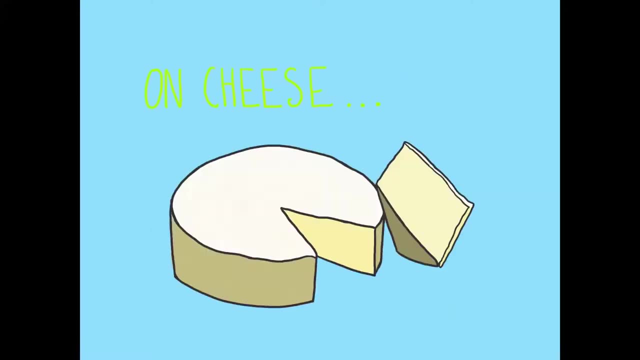 which can be removed mechanically by brushing your teeth. They also form on the surface of ponds and on rocks as pond scum. Biofilms are also used when making cheese. The biofilms are also used when making cheese. They also form on the surface of ponds and on rocks as pond scum. Biofilms are also used when making cheese. 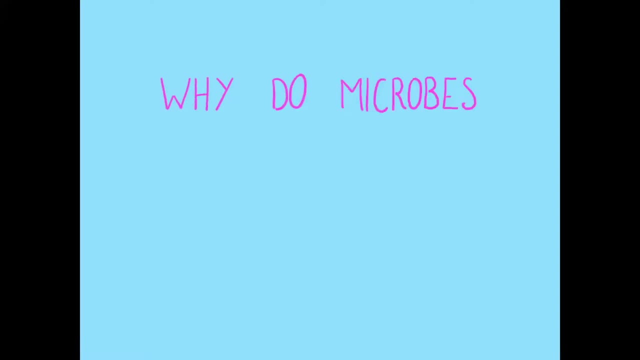 They also form on the surface of ponds and on rocks as pond scum. Biofilms are also used when making cheese. But why do microbes form biofilms anyway? Simply put, there's safety in numbers. The EPS protects bacteria against harsh UV rays from the sun. 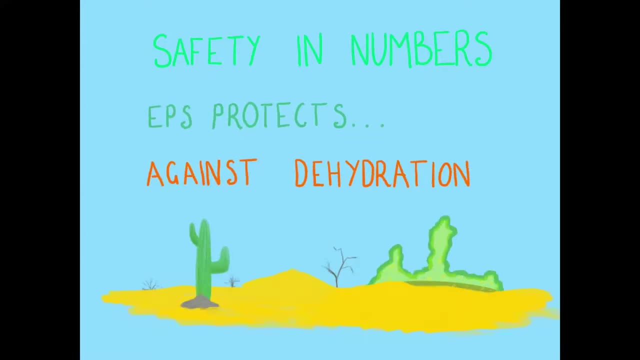 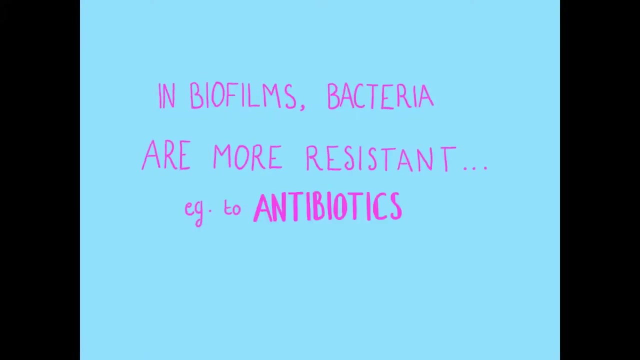 The EPS also helps to protect against dehydration in the case that the biofilm is left exposed. Predators can also be deterred by microbes when a biofilm has been formed. Overall, when in biofilms bacteria are more resistant. For example, most biofilms are antibiotic resistant. 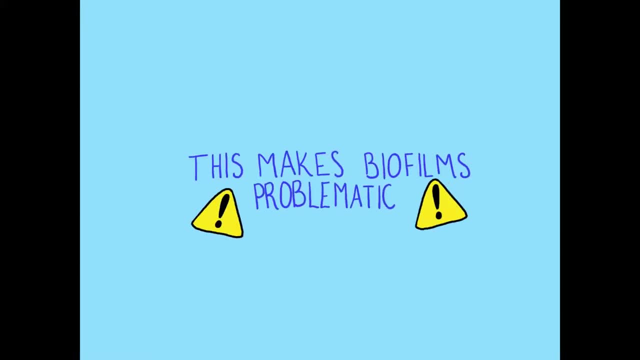 The durability of biofilms makes them rather problematic. For example, if they form on medical devices or implants, they can cause serious infections. They also corrode and block pipes, and can even make your clothes smelly. It is estimated that up to 80% of chronic infections are caused by 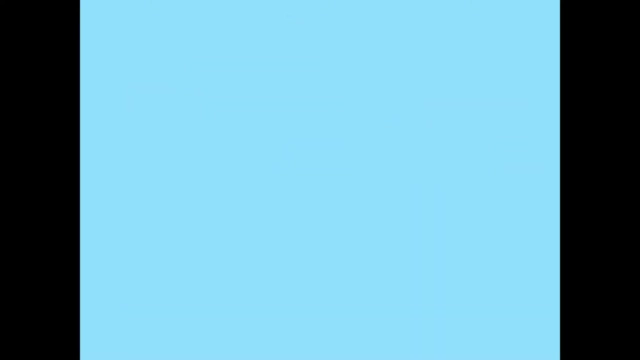 biofilms. Clearly, biofilm formation is a real issue, so one branch of biophysics research aims to manage and prevent biofilm formation. An example of this research is a collaboration between vets and biophysicists at the University of Edinburgh. 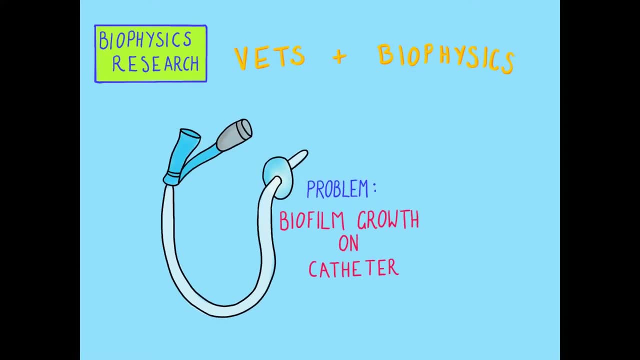 After a catheter implant, animals often develop infections due to a biofilm growth. The team is trying to model the biofilm growth through computer simulations in order to understand and prevent its formation. But it's not all bad. Biofilms can be used to make a positive impact too. 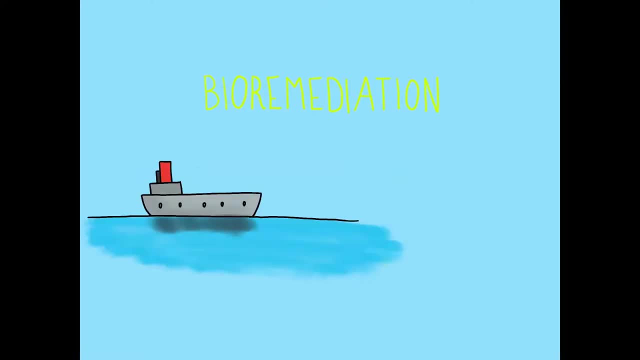 One example of this is in bioremediation. If an oil tanker has an oil spill out at sea, specific biofilms may be grown on the water that actually eat the oil. The microbes digest the oil and turn it into harmless gas and water- Another branch of current